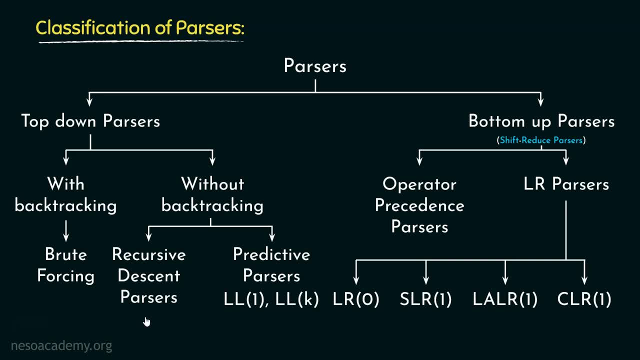 about the recursive descent parsers, didn't we? However, we didn't really go through why it is named like Recursive descent parsers. We have seen how it works- Basically- all the non-terminals are converted into respective functions- and how the entire parse tree is. 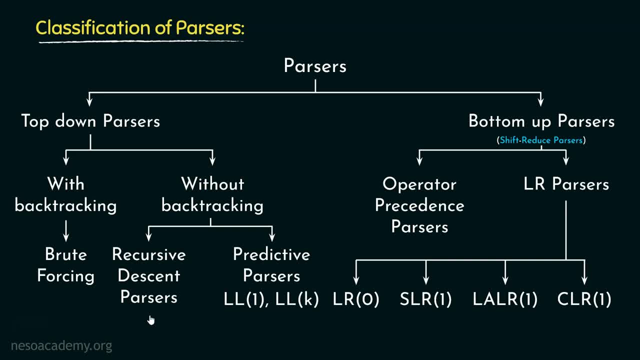 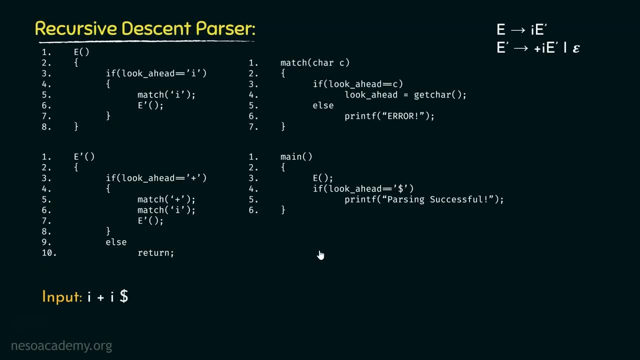 being created Yet again. we don't really know why it's named like this, So let me clear that out for you. So, basically, this was our code for our recursive descent parser. if you remember, The following is one of the main features of this parser- Professor, and he told us that. 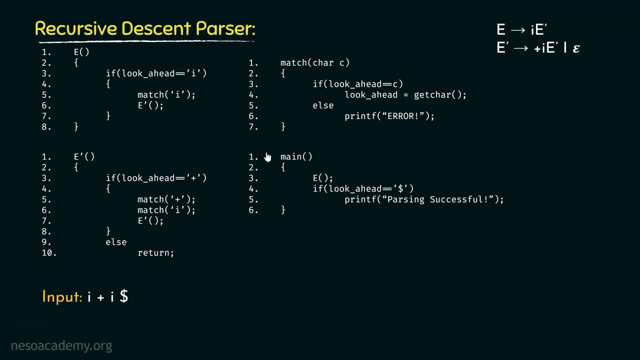 during the classification of parsers, you can only passprefer if the function value exists under the function . So basically, the rect grain written in the rotor equal to �. But now we will know vaya мер function. This is the MATCH function, which helps us with the terminal symbols. This is 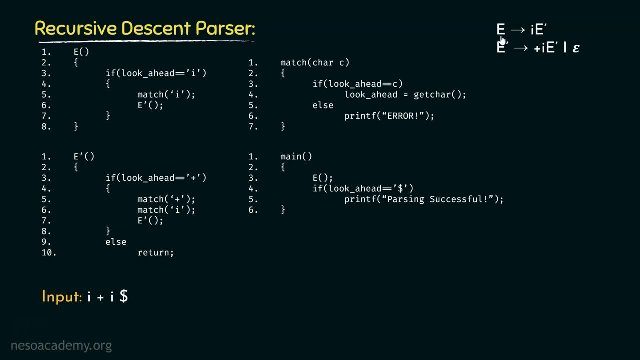 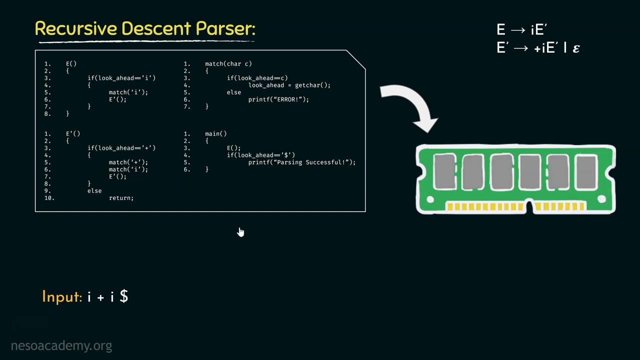 the function e, which mirrors the start symbol of the grammar, And this one here is the function e prime or e dash, which happens to be a mirror image of this non-terminal e dash. Now, when this particular code is placed into the primary memory for execution, it doesn't really remain. 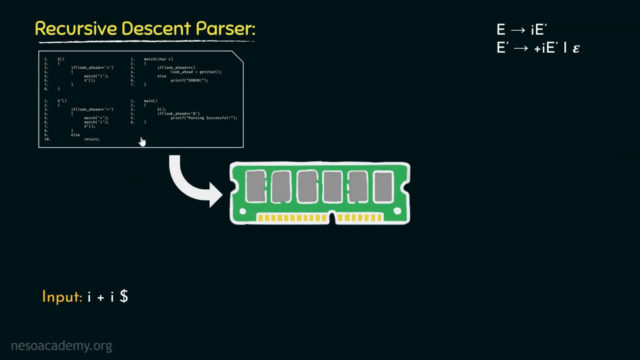 a code anymore. that means a program anymore. Now, this one is a C program, isn't it So in the memory, when it becomes the process, it will have the memory layout as this one. Now, the detailed concept of the memory layout of C programs has been taught beautifully in C programming. 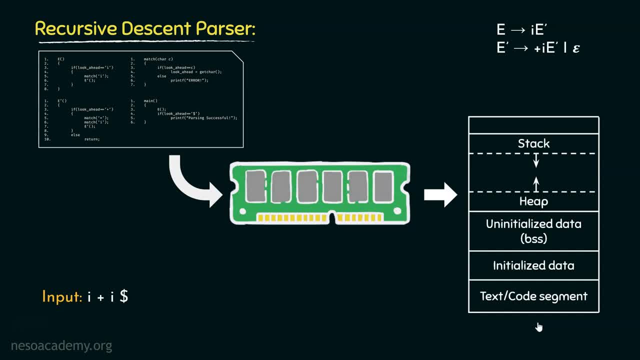 course. So I recommend you all to go through the C programming important question, set 3, for the detailed study of that. Now, in this particular session, we are going to use only the 3. Things which will be useful for this course of compiler design. However, if we briefly discuss, 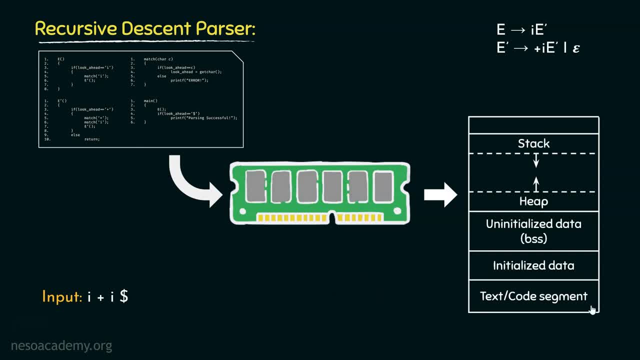 the segments. this is the text or code segment where the code actually resides. Now, coming to the next one: here, the initialized data, that is, the initialized variables, are kept. Now, on top of that, we have the segment for the uninitialized data, which is also called the BSS, Now coming. 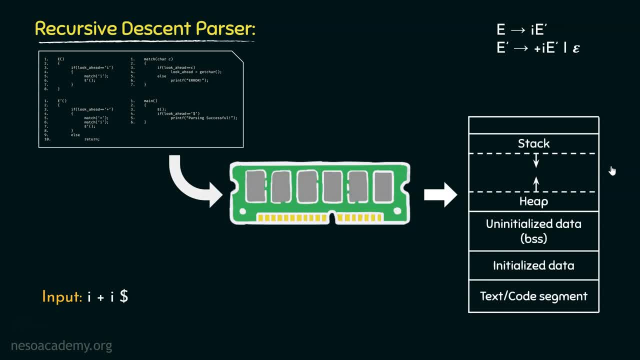 to this segment. this is an interesting one. Here we have both the things: the stack and the hip. Now the stack grows downwards, whereas the hip it grows upwards. Now for the better understanding of recursive descent parser, we actually need this stack Because this particular stack is used. 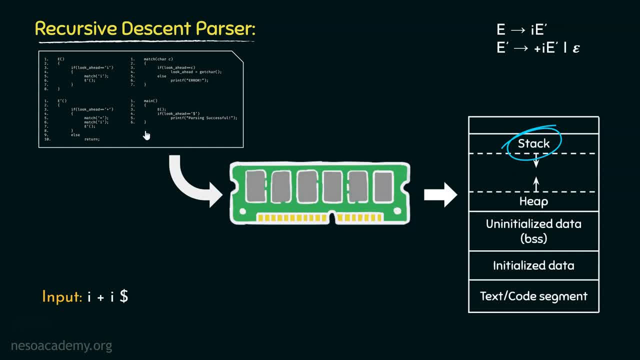 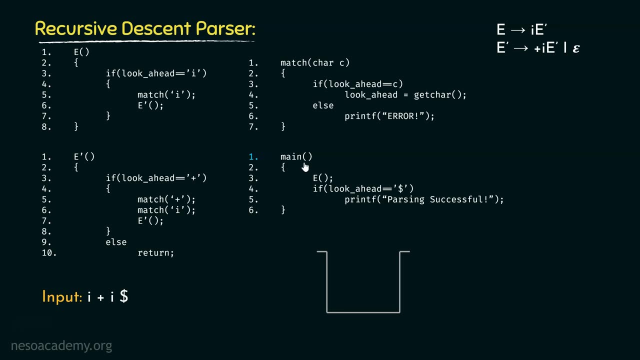 while the execution of the entire program code. Now, logically speaking, the working principle of a stack can be better illustrated with a structure like this one, So we are going to use this one. Now, at this particular line, we already have started the execution of main. So. 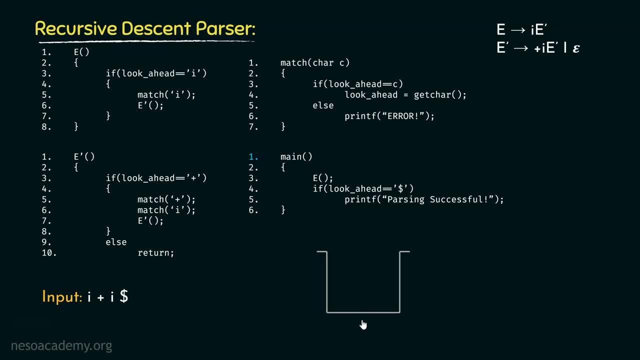 the execution of main starts. In the stack, the activation record of the function main is kept. Now we are going through the main function And eventually, when we hit the line number three, we get to call the function e. Now the calling of the function e signifies the construct of the. 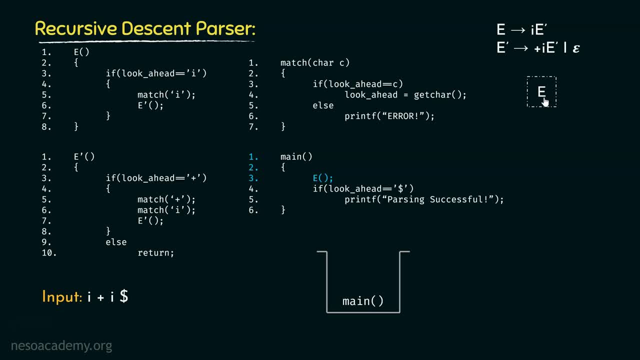 non-terminal e. that is the start symbol in the parse tree. Meanwhile, in the stack on top of the activation record of the main function, the activation record of the function e will be kept Now in the main function. once the execution of the function e is done, the control is going to return at the line number. 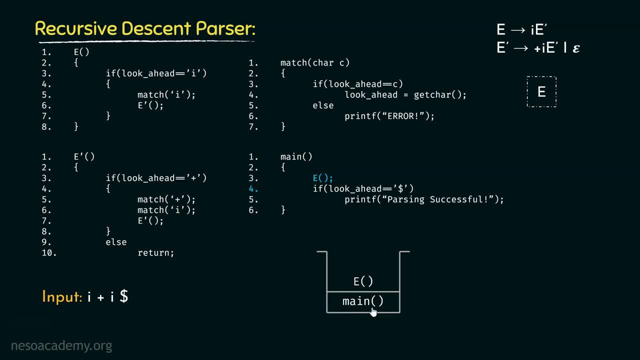 four, isn't it? So in the activation record of main, the operating system will store the line number four, which will be at the anchor point for the function main. Now let's begin the execution of e. So we are in line number one in the function e. Eventually we get to the line number two. 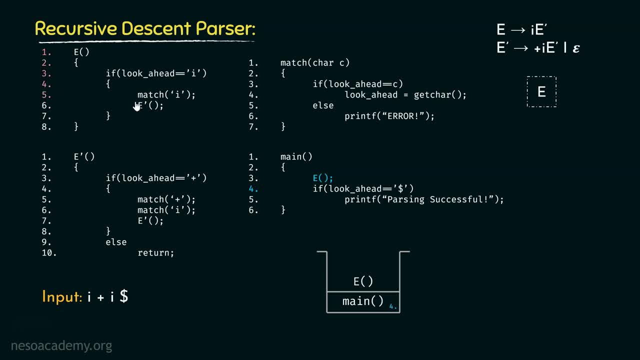 three, four and finally, at five, we get to call the function match i. Now, when match i is called in the stack on top of the activation record of the function e, the activation record of match i will be placed now And the successful execution of which will. 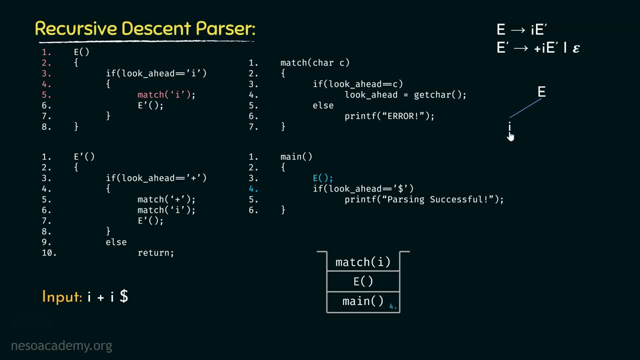 signify the parsing of this particular terminal symbol i in the parse tree. Now, after the execution of match is done in the function e, we are going to return to the line number six. Therefore, in the activation record of e, the operating system is going to store the line number six. 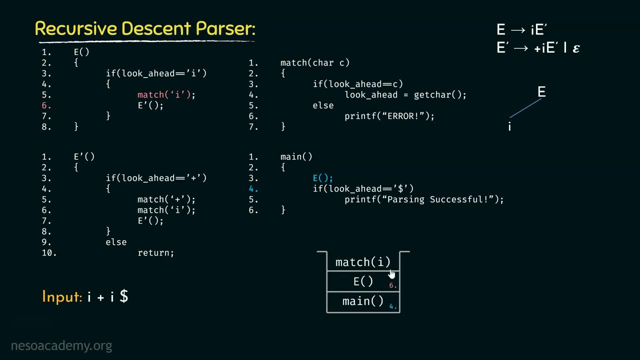 as the anchor point Now say: the match i has successfully executed and we have returned to the function e's line number six. Here we are going to call the function e', aren't we? When the function e' is called, by that time the match i has also been executed. 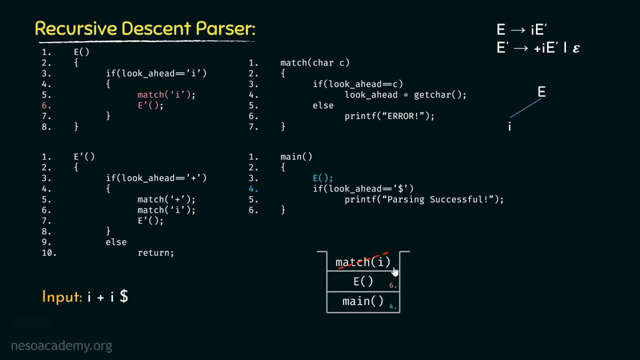 So the operating system is going to pop this activation record and, in place of this one, the activation record of the function e' will be kept, which, if executed successfully, will ensure the derivation of the non-terminal e' in the parse tree. 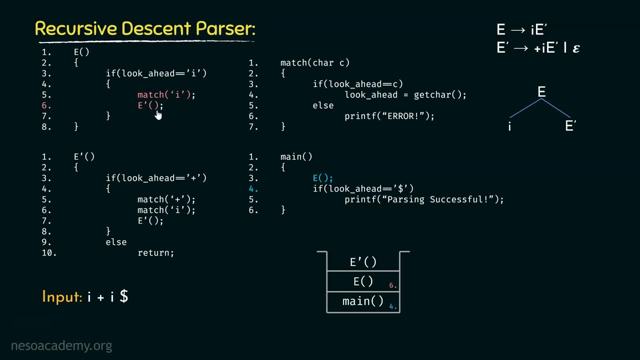 Now, before the execution of the function e' starts, the operating system will notice that the function e will return in the line number seven after the successful execution of the function. e' Isn't so, Therefore, in the activation record of e it will update the. 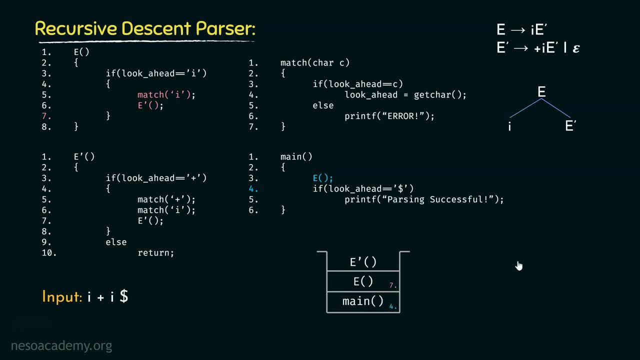 anchor point as line number seven now, And this way the execution will follow. Now, this stack write here is called the recursion stack And it is indeed a top-down parser, And in case of top-down parser, from the start symbol we basically descend in order to generate the. 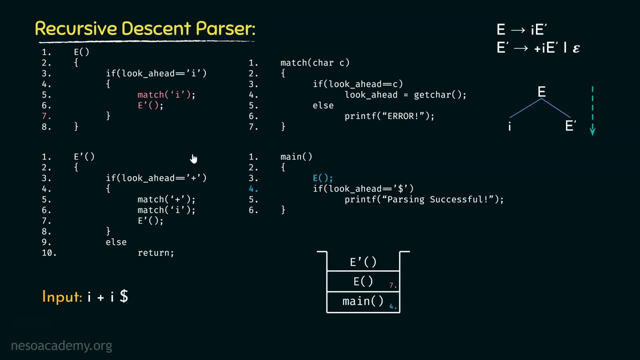 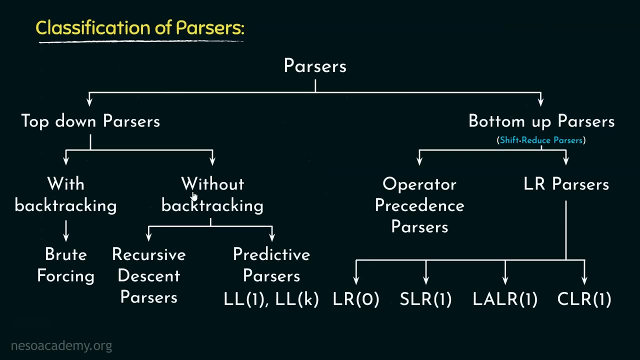 parse tree for the input stream And that's the reason why it is called recursive descent parser. Remember, we are using a recursion stack and, due to top down parsing, we are basically descending, Hence the name recursive descent parser. Now in this session, 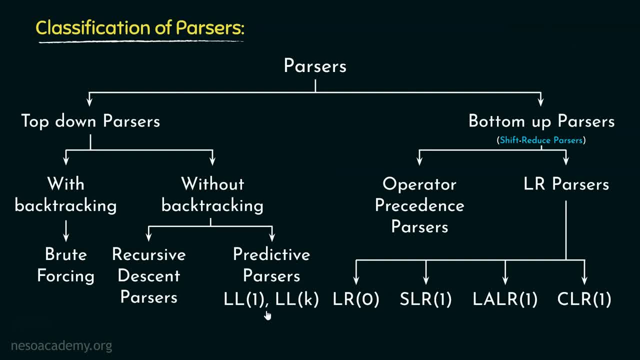 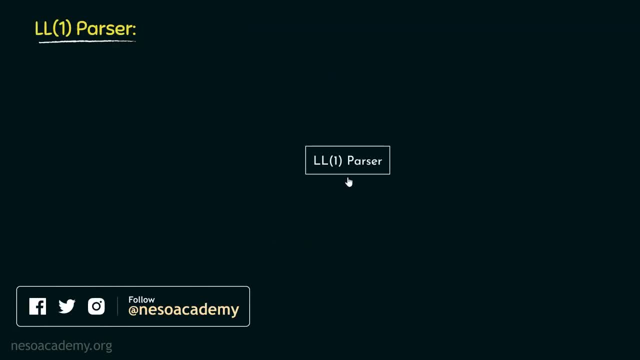 are going to start learning about the predictive parsers, that is, LL1 parsers, Now coming to LL1 parsers. for the construction of the LL1 parser, we will need a few components. First we will need an input buffer, basically where we will store the input. Now, if you remember, the inputs are: 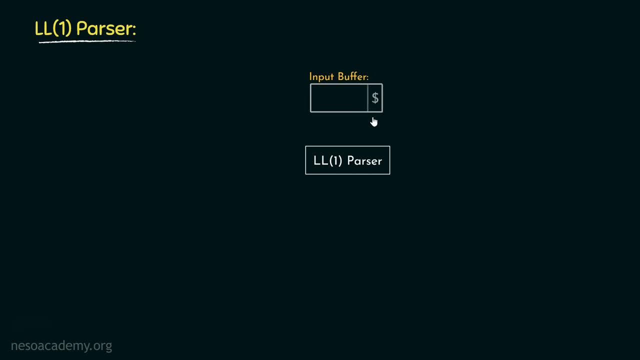 always kept with the dollar symbol by the end, So let's place the dollar symbol in here for better significance. Now, from the input buffer, the LL1 parser will receive the inputs, naturally. Now for the construction of the parse tree LL1 parser will need something called an LL1. 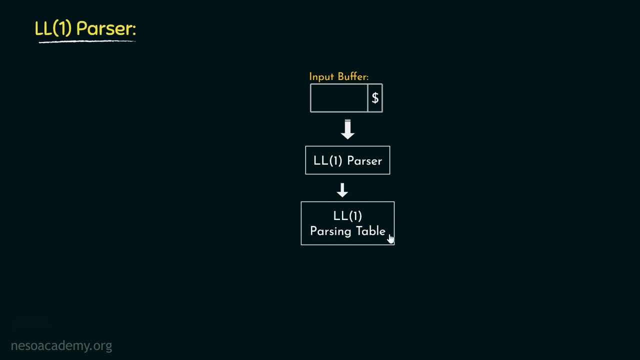 parsing table, And once this has been created, after that the LL1 parser will use the elements from this one during the construction of the parse tree. Now, alongside the input buffer and the LL1 parsing table, the LL1 parser will also need the stack And the bottom of the stack. 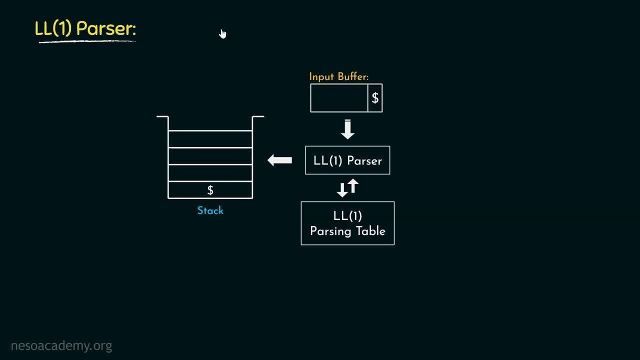 will be denoted by the dollar symbol. So this is the organization of the LL1 parser. Now, since we have already seen it, let's move on to the name of the LL1 parser. Now, the first L in LL1 parser. 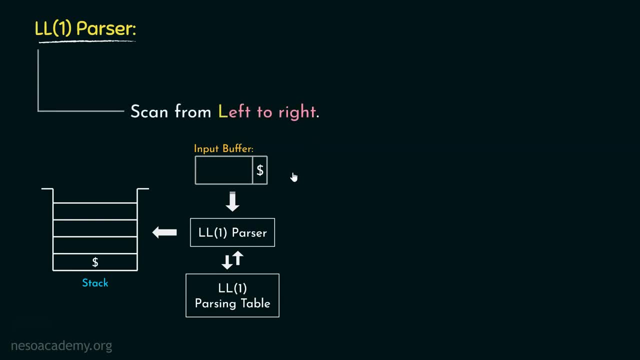 stands for scan from left to right. Try to understand this. This is the input buffer And here the strings will be kept While we proceed with the LL1 parsing, the input streams will be scanned from left to right. So this L signifies that 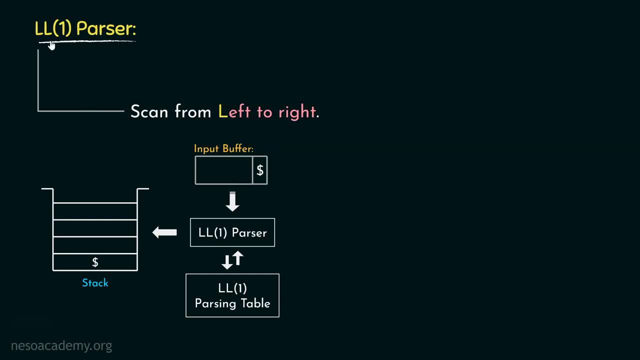 Left to right of the scanning. Coming to the next L, I hope you all remember that it is a top-down parser And all the top-down parser uses top-down approaches, And top-down approach uses leftmost derivation. Hence, the next L signifies the use of leftmost derivation. Now, coming to the one in 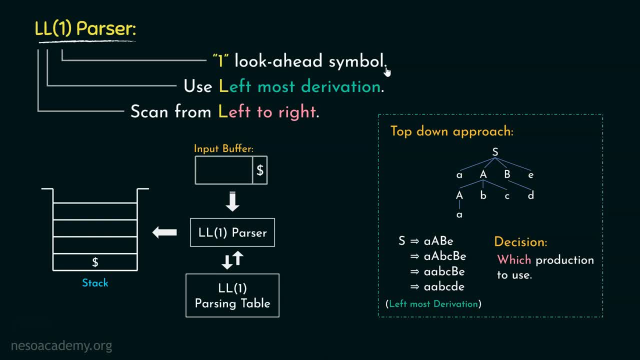 here, it specifies one look-ahead symbol. Now, if you remember, LL1 parser is a type of predictive parser. Focus on the name: predictive. Basically, the LL1 parser will generate the parse tree, taking decisions from the LL1 parsing table based on one look-ahead. 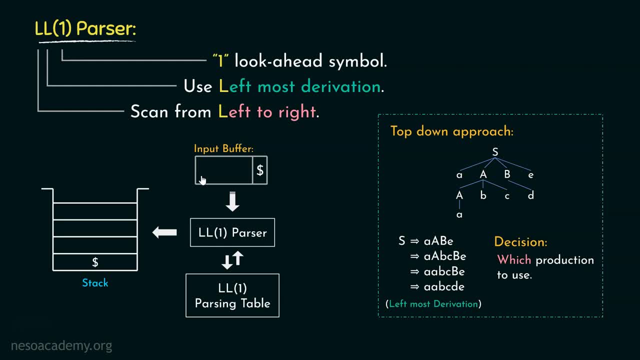 symbol from the input buffer in every iteration. So this is how the LL1 parser gets its name. Now, before we learn about the LL1 parsing method, we need to learn how to construct this LL1 table. And in order to construct LL1 parsing table, we need to learn about two different. 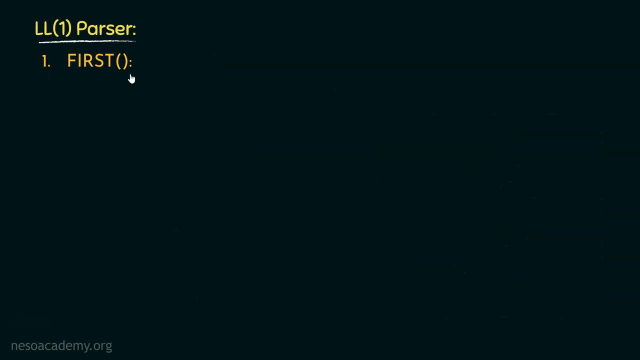 concepts. Coming to the first one, that is the first function. Now what is first Given? any non-terminal of a CFG, that is a context-free grammar if we derive all the possible strings from it. the first terminal, or terminals, is the first of the non-terminal. Let me explain with: 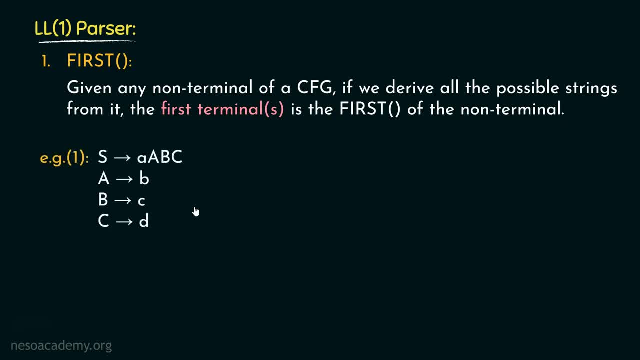 an example. See, this is a context-free grammar. S can be rewritten as small, a capital A, capital B, followed by capital C. Now let's try to find out the first of S Now from this particular production rule, from S, we can derive this: 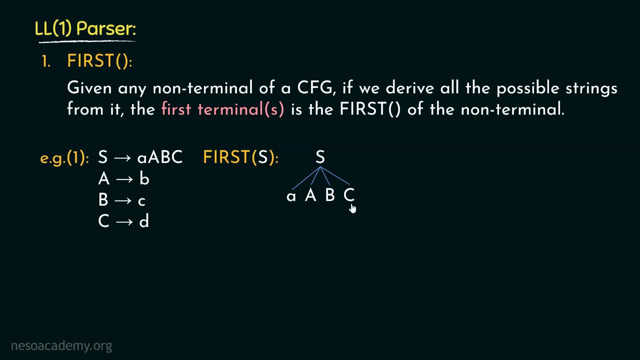 A, followed by capital A, capital B, capital C. Now, this is the only string which can be derived from S according to this particular grammar. However, the first terminal in this particular string is this small a. So the first of S is going to be this small a. Now observe, given any non-terminal of a CFG. 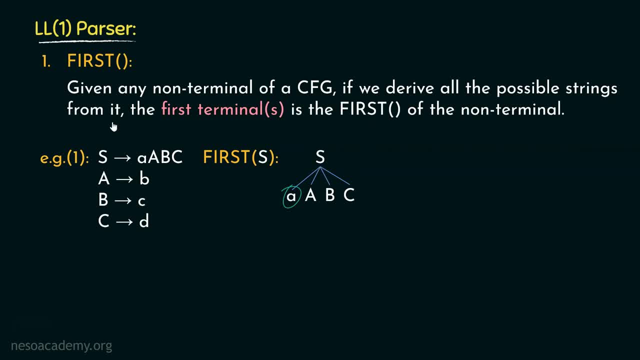 that is this non-terminal, if we derive all possible strings from it. unfortunately, this is the only string which can be derived from here. Anyway, this will stand for now. The first terminal is the first of the non-terminal, So this is the first terminal. Therefore, this is going to be the 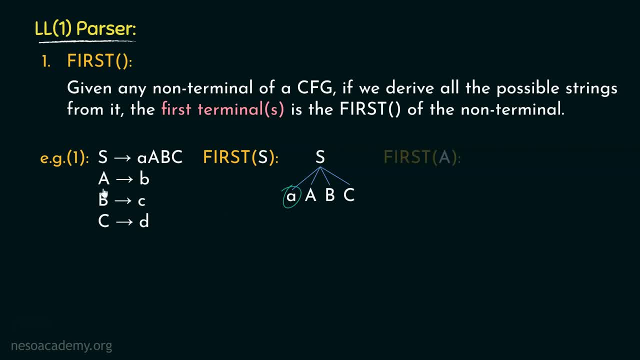 first of this non-terminal, The first of A. Let's do that Now. from A we can only derive the terminal symbol B. So this is going to be the first of A. What will be the first of B? Now, from B, we can derive C, following this: 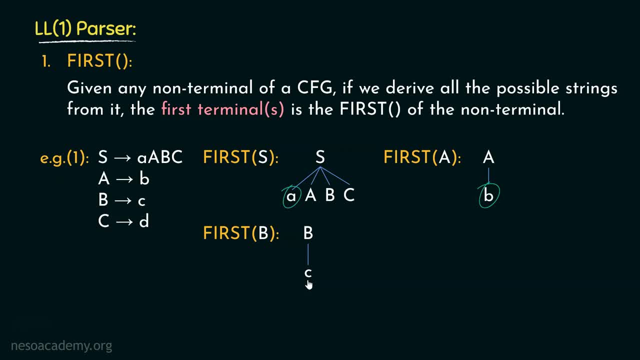 production rule B can be rewritten as small c. Therefore this is the terminal, which is going to be the first of this non-terminal B. Now we are only left with C, and C can be rewritten as D, So the first of C, that is, C, can only derive B. 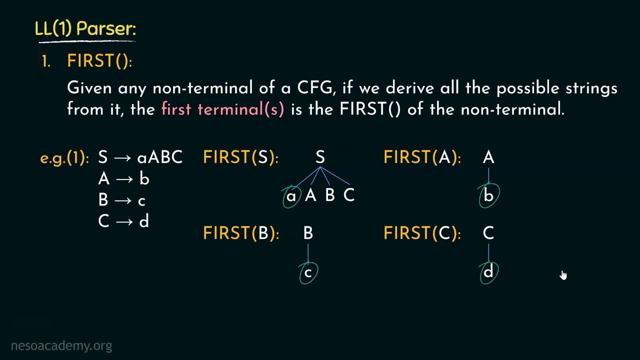 And hence it will be D. only Interesting, isn't it? Let's go through another example. shall we Consider this grammar? Let's find out the first of S. Now, considering this production rule, from S we can derive A, B, C. Now, these are all non-terminals. In case of first, we need the 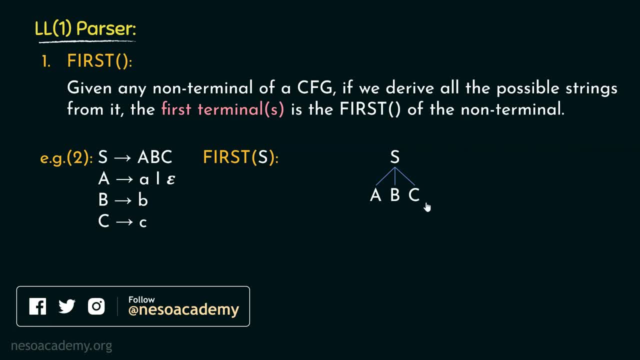 first terminals. Now, coming to this string, this is the first non-terminal And using this production rule, that is, A can be rewritten as C. So this is the first non-terminal. Now from A we can derive A. So if we derive it like this, in that case from A, the first terminal. 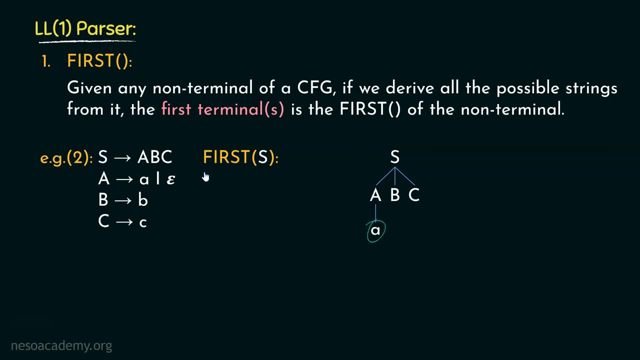 that we get is small a, So in first of S small a will be there. Now there is another production rule involving the capital A, That is, A can be rewritten as epsilon. So if A derives epsilon, this will signify that we haven't derived any terminal symbol yet. So now we have to consider. B. Now from B we can derive A, So from A we can derive A. So if A derives epsilon, this will signify that we haven't derived any terminal symbol yet. So from A we can derive small b. 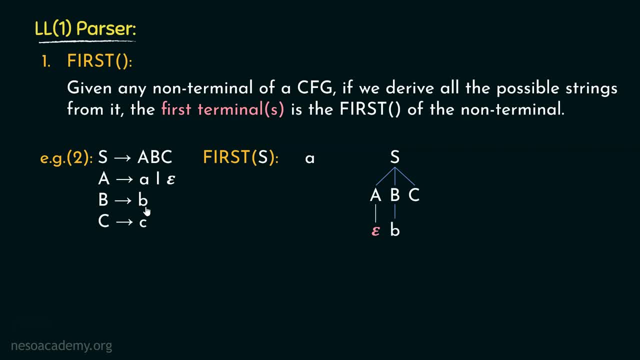 Following this production rule, B can be rewritten as small b. Therefore, if A derives epsilon, in that case for S, the first terminal that we will derive is B. Therefore, in first of S B will also be there. So these two terminals will be included in the first of S. Now observe: 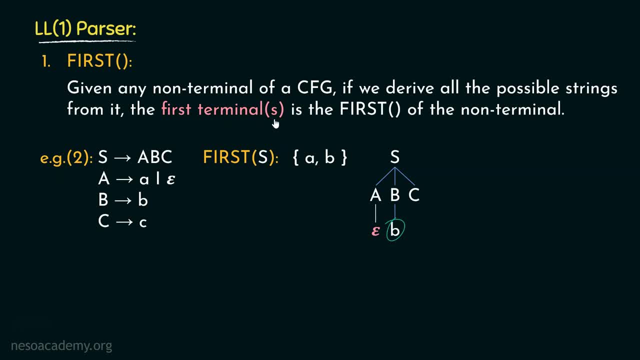 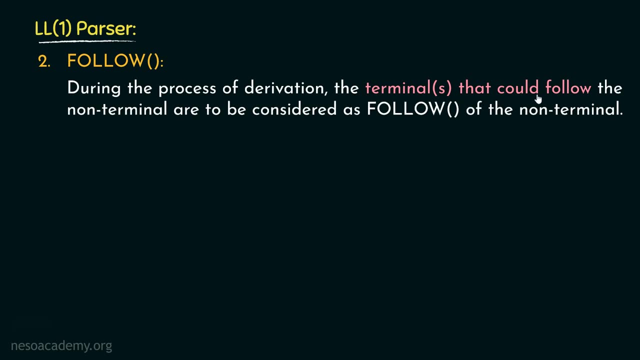 we already mentioned, it can be a terminal or a set of terminals, didn't we? So this is the set of first. Let's move on to the next one, that is follow. Now, follow is during the process of derivation. the terminals that could follow the non-terminal are to be considered as follow. 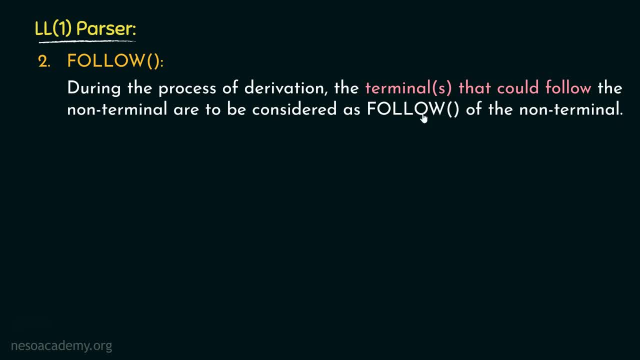 of the non-terminal. Basically, all the terminals which will follow the non-terminal will fall under the follow set of that particular non-terminal. Let me illustrate this with an example. Observe this grammar: Here the start symbol is S. Now if we talk about the follow of S, apparently S is not being followed by anything. However, 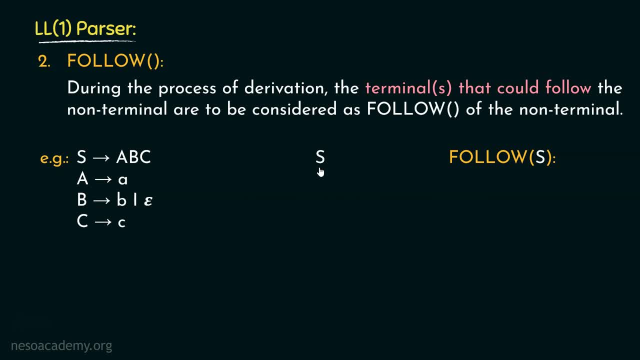 if you remember, the derivation will always start from the start symbol S itself, and both in the input buffer and in the stack, which will be followed by the dollar symbol. So, basically, the start symbol is always followed by the dollar symbol itself. So in the follow of S, 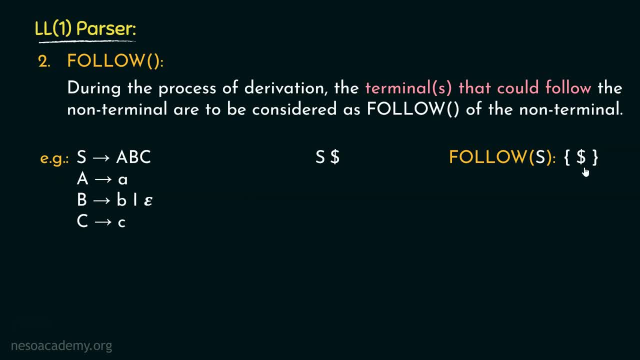 that is the start symbol. we will at least have the dollar symbol Now. from the start symbol S we can derive A, B and C using this production rule, can't we? Let's now find out the follow of A. 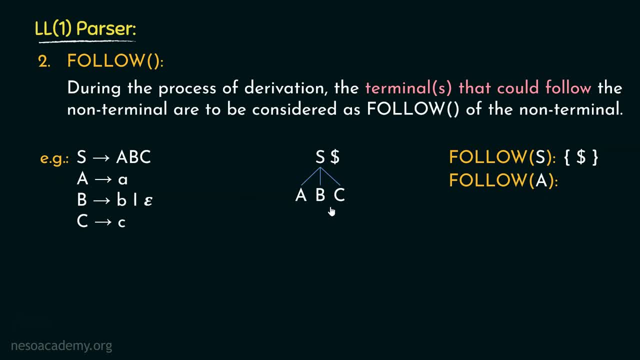 Now observe: the non-terminal A is followed by BC. These two are also non-terminals, But in the set of follow we need terminals. Now, coming to B, it can derive B, that is the small b. So basically, during the process of derivation the non-terminal A is actually followed by. 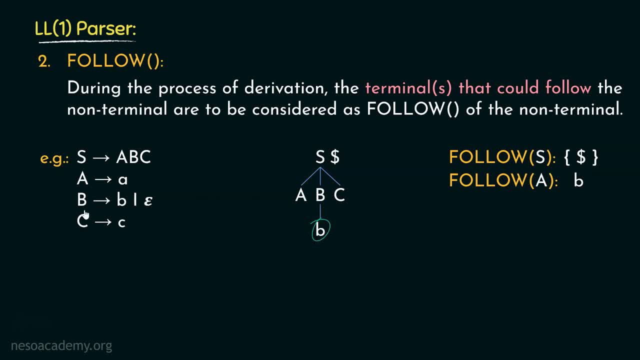 the terminal symbol B. There is another production rule involving the capital B, non-terminal, that is, B, can be rewritten as epsilon. So in case B derives epsilon, in that case we don't have any terminal yet which will follow A, So we need to consider C now. 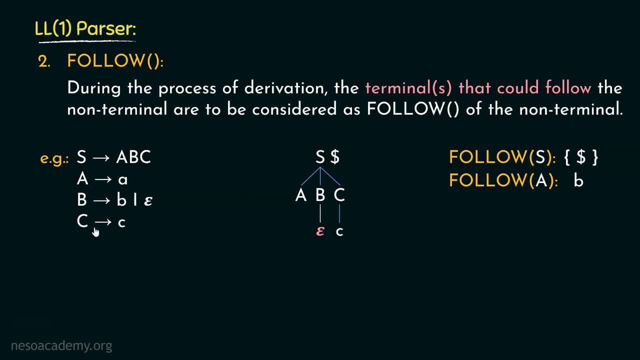 Now C can derive small c. using this production rule, C can be rewritten as small c. So in case B derives epsilon, in that case the non-terminal A is being followed by the terminal symbol small c. Therefore, in follow of A we will have the terminals B and C. 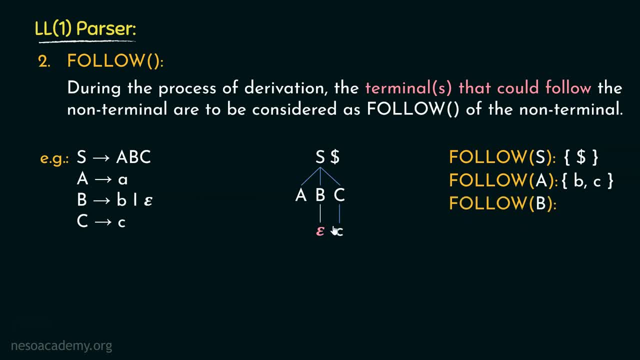 Let's now find out the follow of B. Observe B is being followed by the terminal symbol C. Hence the follow of B will have the terminal C. Now, what about the follow of C? Although it may look like C is being followed by nothing, but, if you remember, S was being 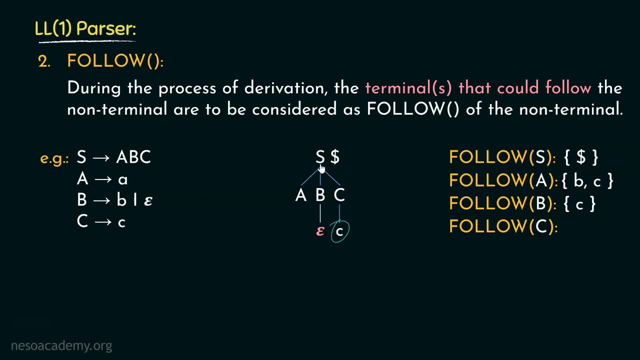 followed by dollar symbol, And While s got replaced by this string, a, b, c, c became the rightmost symbol, which should also be followed by the dollar symbol. Therefore, the follow of c will have the dollar symbol. So basically.